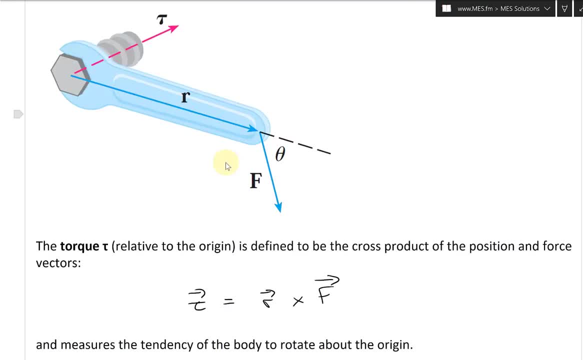 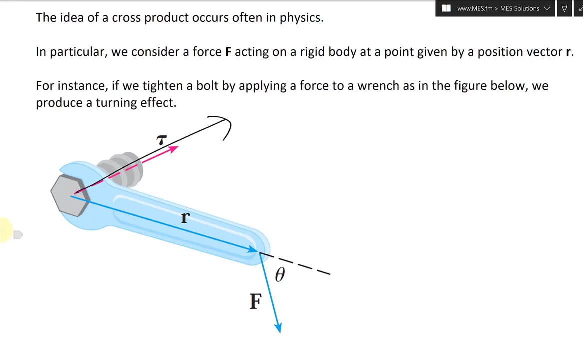 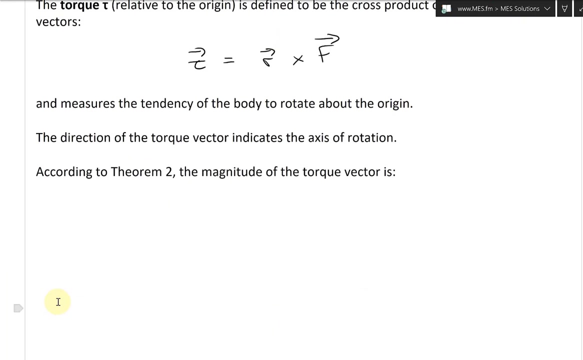 of the torque vector indicates the axis of rotation. So if it's pointing here, and then if you're doing right hand rule, this would be curling. see how this would be. this would be curling downwards. So right hand rules this way, your fingers are curling inwards this way and you're right in your thumb sticking up Again, just using the right hand rule like that. And then, according to theorem two, the magnitude of the torque vector, 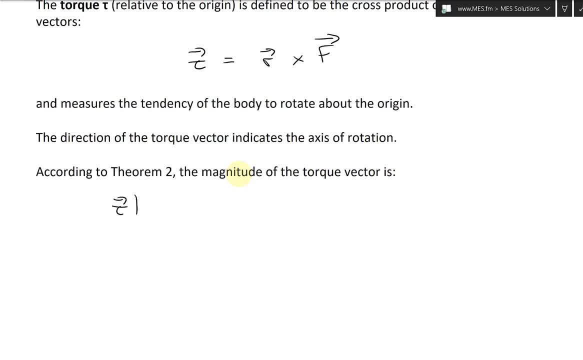 is, and again, the absolute value, or the length or the distance, or just the magnitude of the torque is equal to the magnitude of the cross product of r, cross f, which equals to the magnitude of both position vector and the force vector, and then sine theta. so there's that sine theta across here. 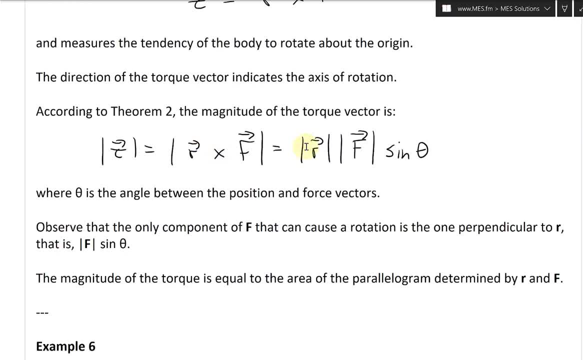 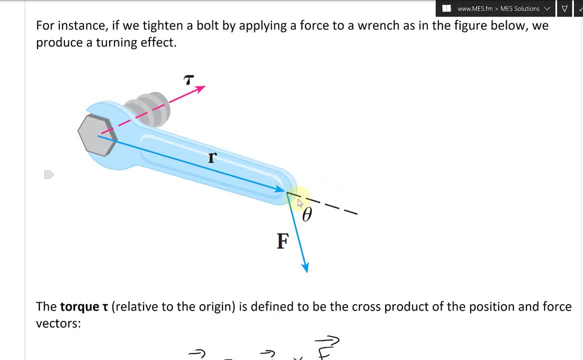 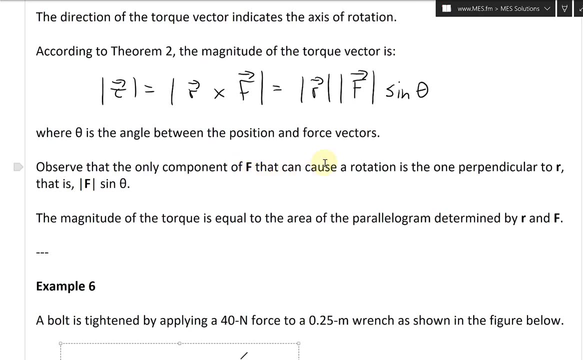 like that, pointing downwards, yes, uh, and where this theta side? this theta is again the angle where. where theta is the angle between the position and force vectors like that. it's fascinating stuff. so now observe that the only component of f that can cause a rotation is the one, uh, perpendicular. 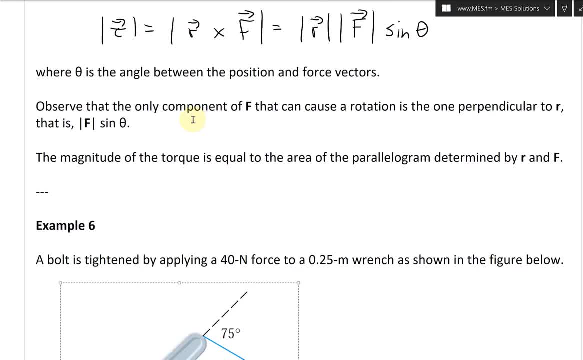 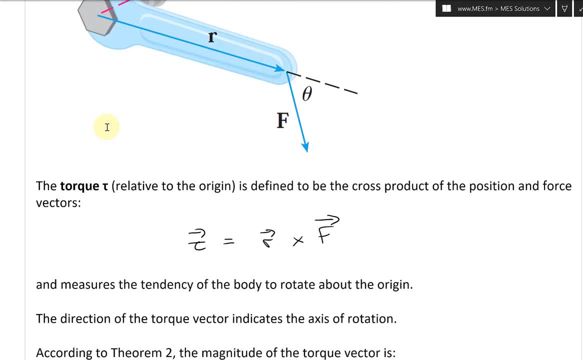 to r. it's the only one you have perpendicular to this and that is again, uh, this, uh, uh, force, uh, the length, the magnitude of the force vector is equal to the angle between the position and force vector to the force times by sine theta. so it's only this component, right here. 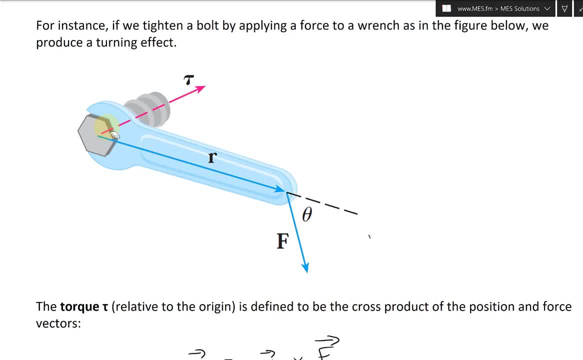 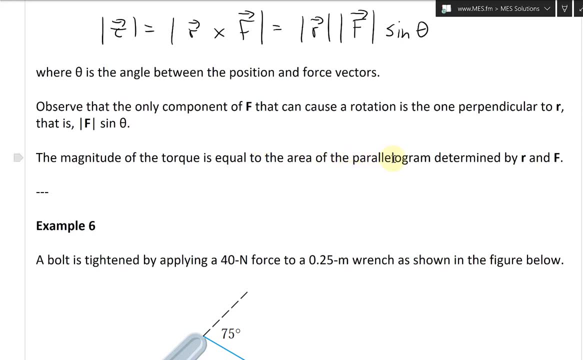 sine theta. perpendicular like that. that's fascinating stuff here. now let's continue further. so and the magnitude of the torque is equal to the area of the parallelogram determined by r, position vector r and the force vector f, again with the um based on the cross product, is just the parallelogram. 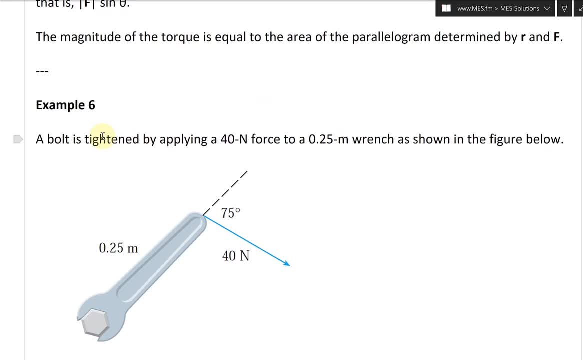 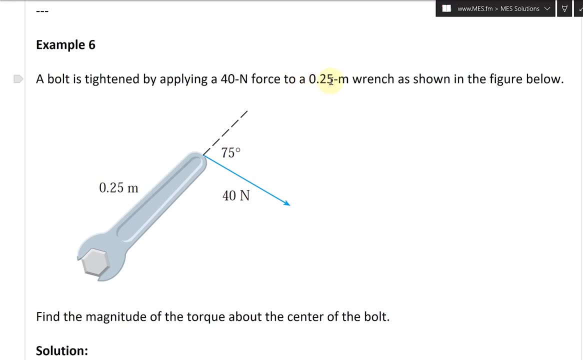 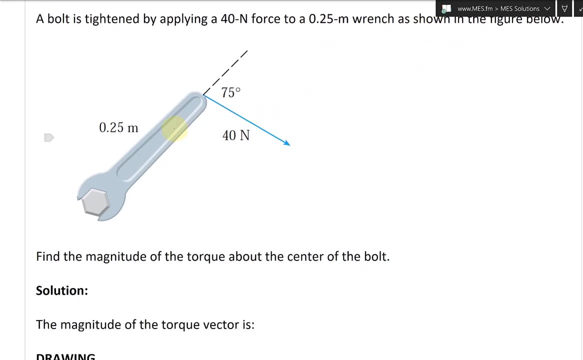 of the two vectors. now let's take a look at example six, the last example of this video. then we'll do the exercises. so a bolt is tightened by applying a 40 newton force to a 0.25 meter wrench, or 25 centimeters, as shown in the figure below. so here's the. you're tightening this one here. 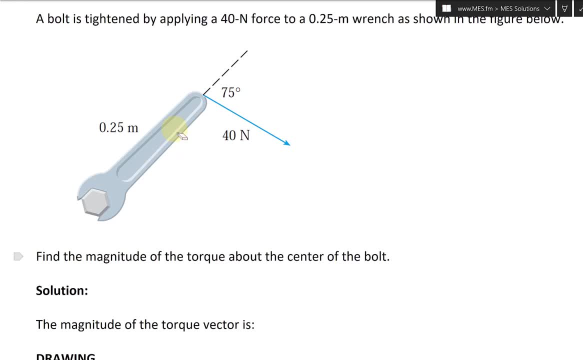 you're doing uh, you're doing clockwise, so your fingers are going inward, yeah, so then the, the, the arrow, is going to be going in into the page, like straight down into the page, like that is your thumb. so that's the torque is going into the page anyway. so there's the 0.25 is the r value, the length of the uh r, and then this is: 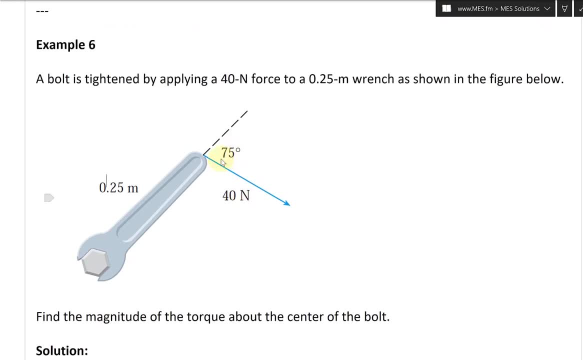 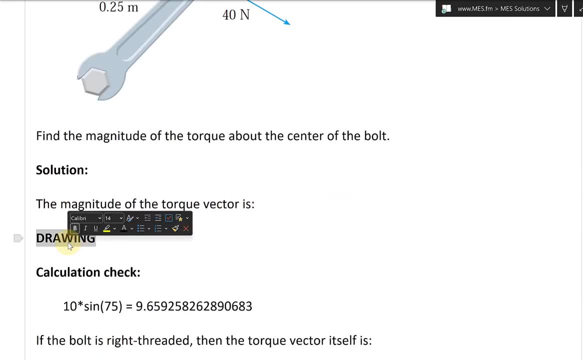 40 newtons is the magnitude of the force, and there's the 75 degrees and it says: find the magnitude of the torque about the center of the bolt. so solution: let's go here, all right. yeah, let's move those over down here. so the magnitude of the torque is going to be the center of the 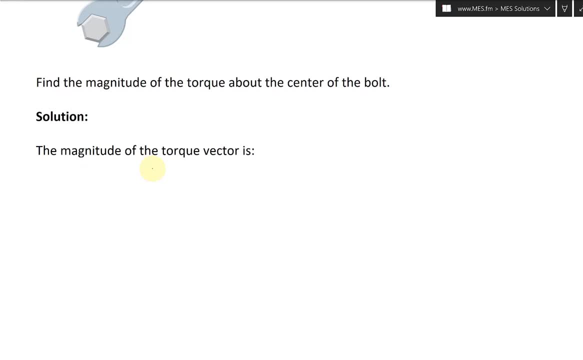 bolt. so solution: let's go here, all right. yeah, let's move those over down here. so the magnitude of the torque vector is: well, we just use a cross product, so this is a tau, this is a torque. the magnitude of the torque, like this, so value sign, is equal to magnitude of the uh cross product r. 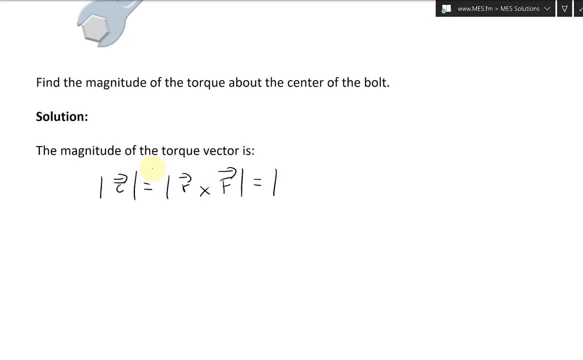 cross f. this equals two using the theorem two. so this is gonna be a length of r times by length of f. this equals two using the theorem two. so this is gonna be a length of r times by length of f. as by sine of 75 degrees. as by sine of 75 degrees. 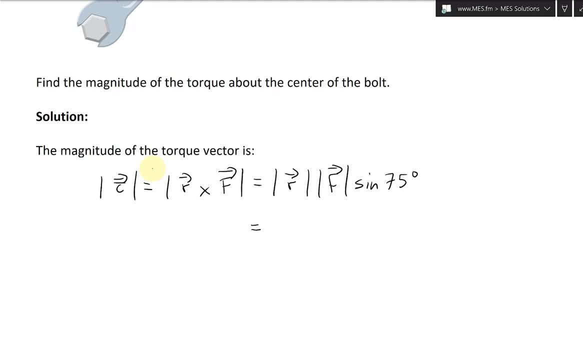 and then, if you plug this in, we'll also put everything in. so the the distance is 0.25 meters, 0.25 meters, and then the force is 40 newtons. see that up here. so 0.25 meters, 40 newtons. 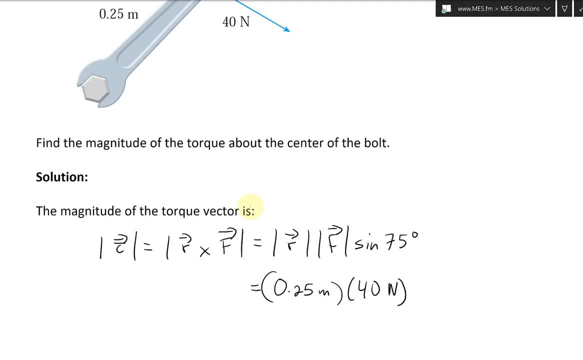 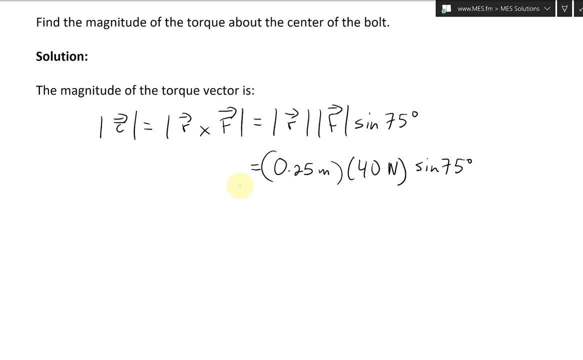 it's gonna be 40 newtons and then sine 75 and then, uh, if you solve this again, this 0.25, that's just 1 over 4 times by 40, that's going to be- um, it's going to be 10 equals to 10 sine 75. let's get this better. 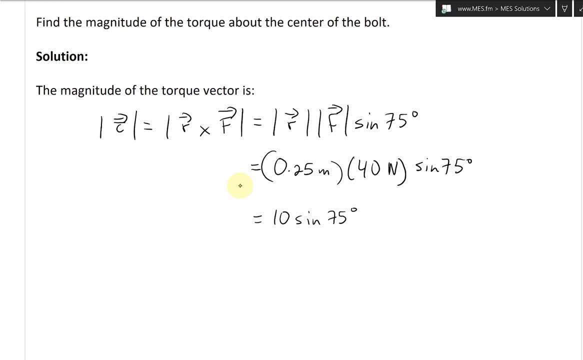 75 degrees, and then if you um, and then now this equals two and this equals to uh, plug in the calculator again. so it's going to be 10 times sine 75 degrees. so we get 9.66 newton meters, and i'll solve this.